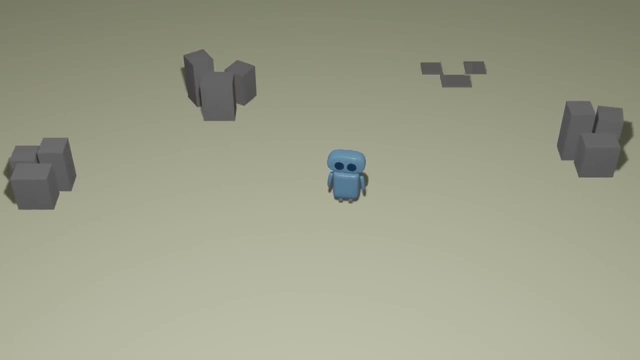 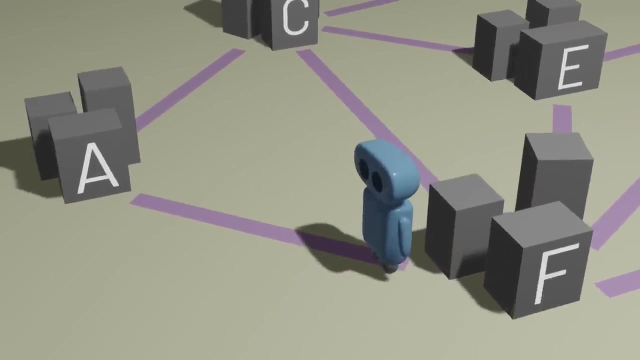 To understand what Dijkstra's algorithm is and how it works, let's start with a scenario. Let's imagine that we have a variety of different towns scattered in different locations. Some of those towns are connected to other towns with roads, such that we could travel along a road to go from one town to another. 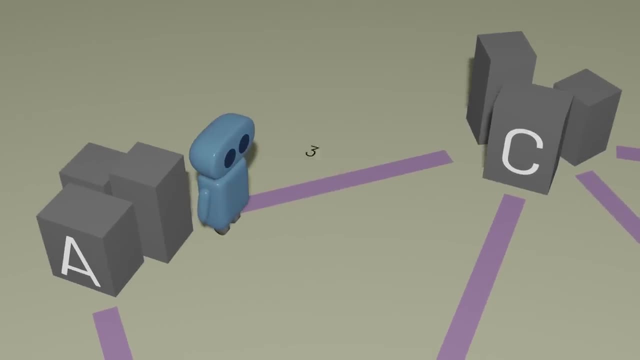 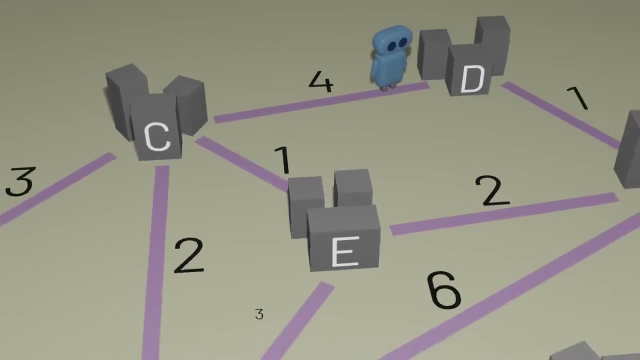 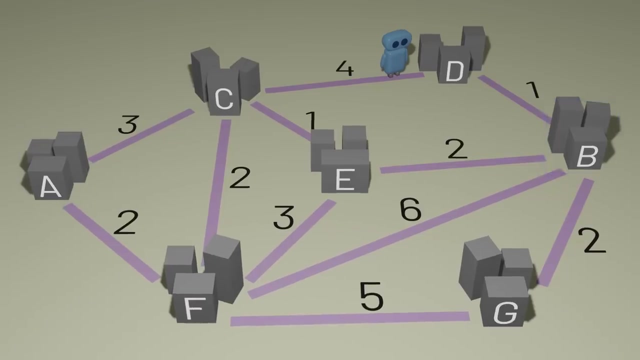 Not all roads have the same travel time, though. One road might take three minutes to travel through, while another might take four, And our question is this: What's the fastest way to get from town A to town B? This is a specific example of a more general problem in graph theory. 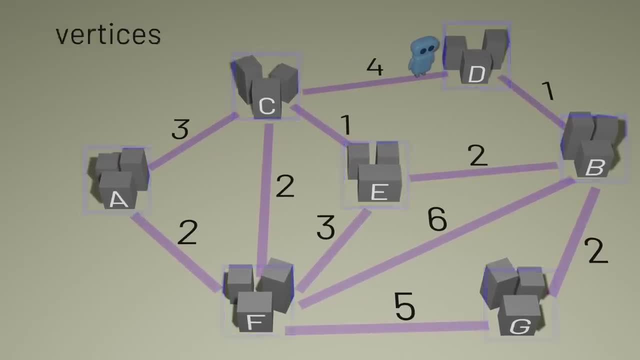 where we have vertices- in this case, our towns- that are connected by edges- in this case, our roads. Together the vertices and edges form a graph And, in particular, this graph is a weighted graph, because each edge has some value or weight. 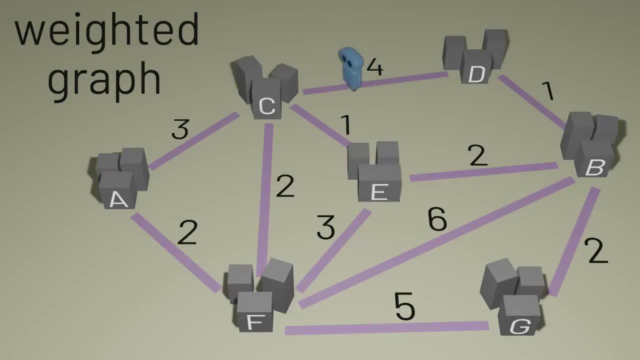 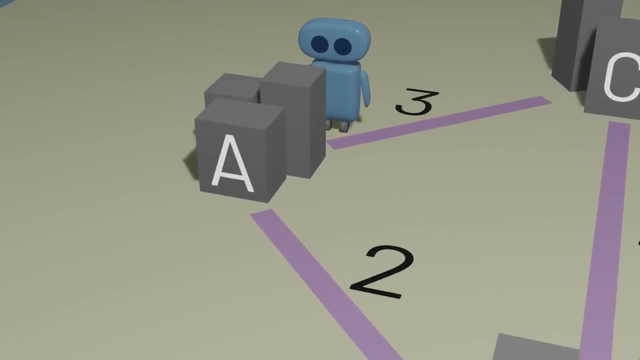 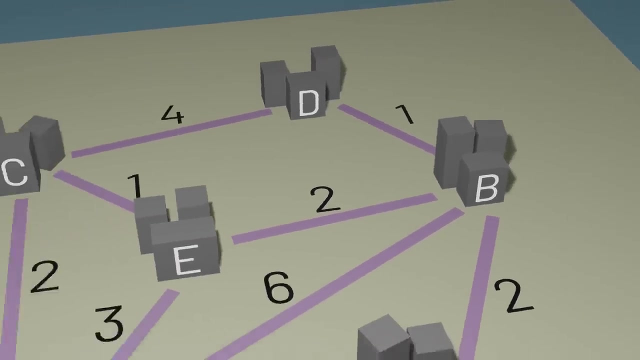 to indicate how costly it is to travel along that edge, measured in either distance or time, And with this graph we'd like to determine the shortest path from one vertex to another. So how does Dijkstra's algorithm allow us to do this? 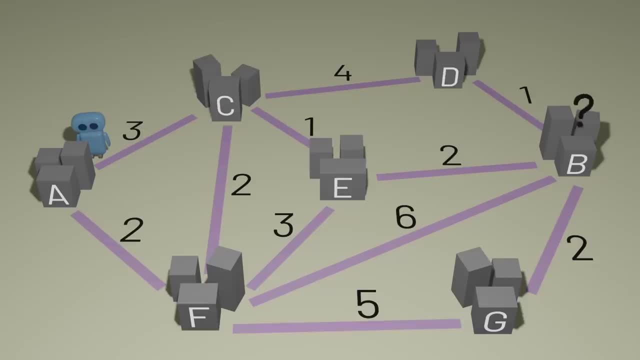 Ultimately, we need to figure out how many minutes it will take to get to town B. In doing so, though, it might be useful to figure out how many minutes it would take to get to the other towns too. So, ideally, we'd want to label each town with a number. 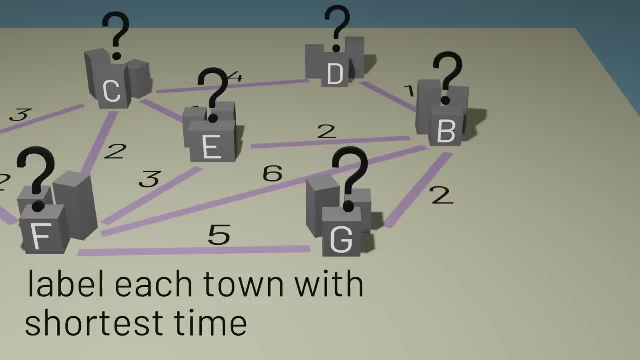 representing the shortest time required to get there, But of course we don't know that information yet, So instead we'll label each town with the shortest time we've found so far to get to that town Before we've started the algorithm. 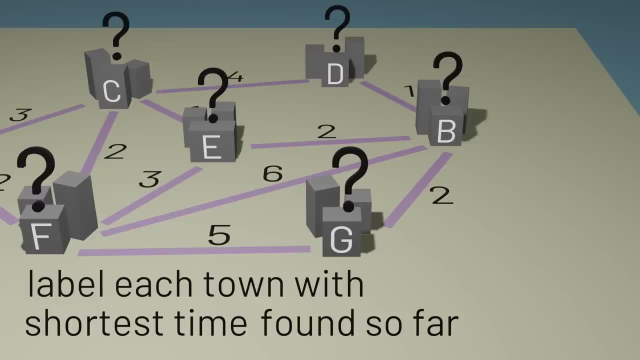 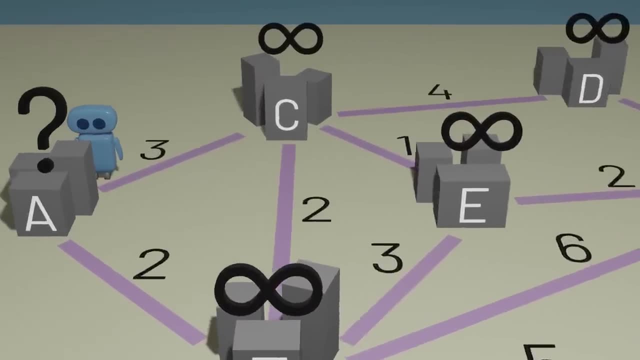 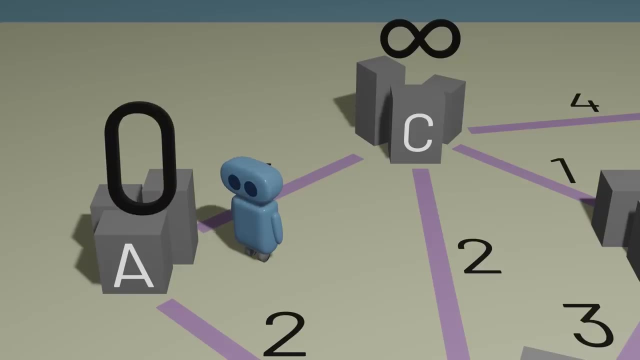 we don't have any known way of getting to the towns, so we'll label them all with infinity. The only town that we can label correctly is our source, town A, which we can easily label. We're starting there, so it takes zero minutes to get to this town. 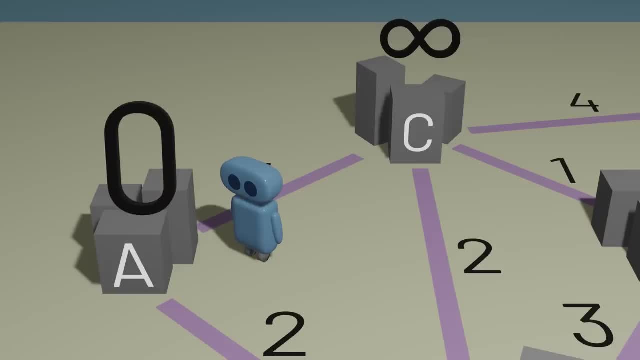 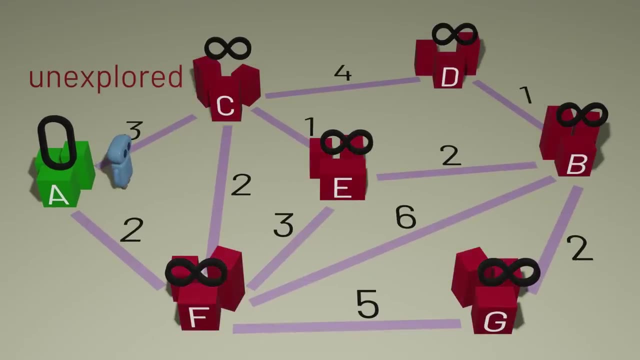 Once we've found the shortest path to a town, let's call that town explored. For all other towns, we'll consider them unexplored. We don't yet know what the shortest path to them is. So what can we do next? 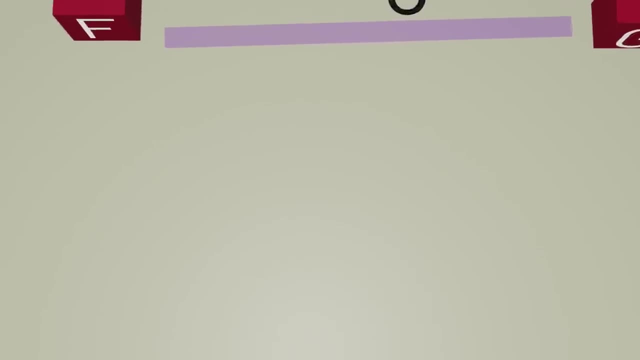 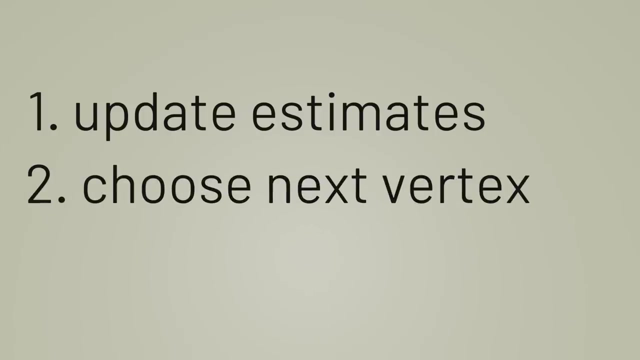 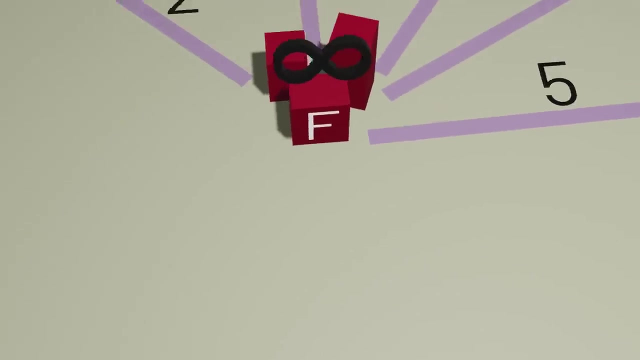 Dijkstra's algorithm repeats a two-step process: First we update our estimates and second we choose the next vertex to explore. So let's start with the first step: updating our estimates. We know we can get to town A in zero minutes. 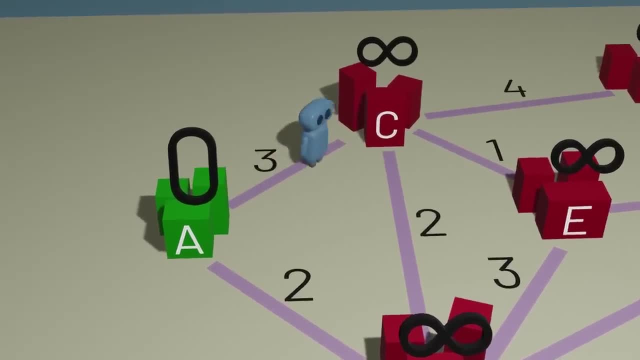 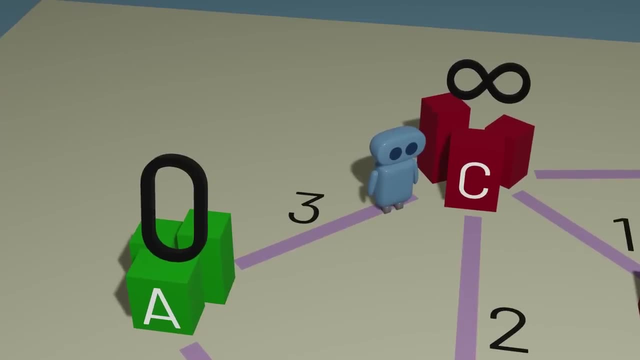 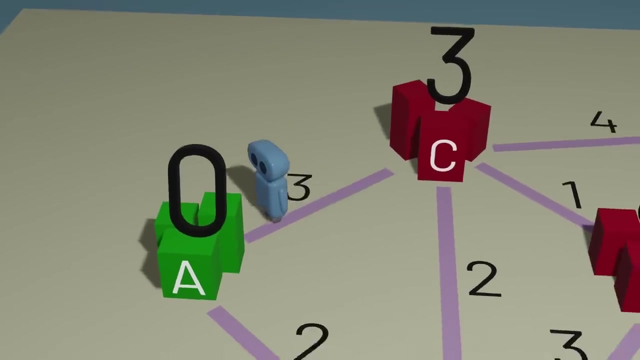 and because we can get from town A to town C in three minutes. we know we can get to town C in three minutes. That's much better than our current estimate of infinity, so we'll update our estimate to be three And we can do something similar for town F. 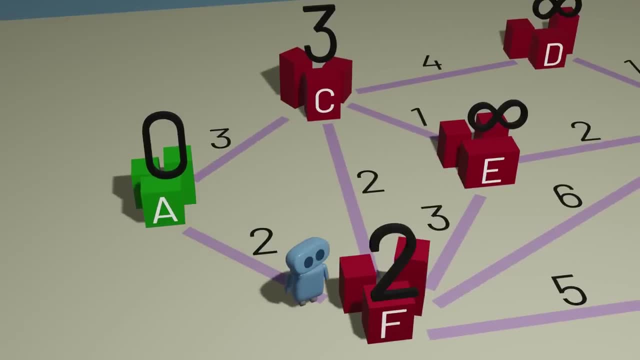 We can get there in two minutes, so we'll update our estimate After we've considered all possible roads connected to town A. we're done with this step, And now the next step is choosing which town to explore next, And the rule is quite simple. 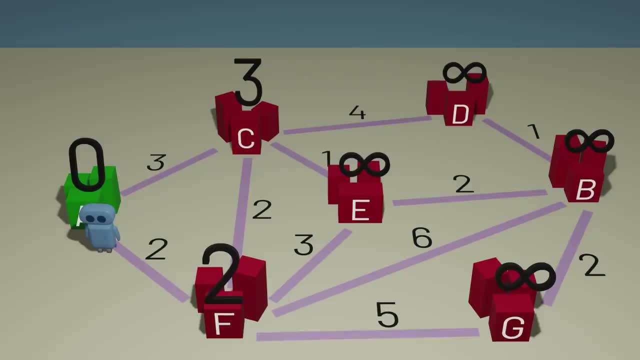 The town we explore will always be the unexplored town with the smallest estimate. In other words, the next town we explore should be, among all of the unexplored towns, the one we know we can get to the quickest. In this case, that's town F. 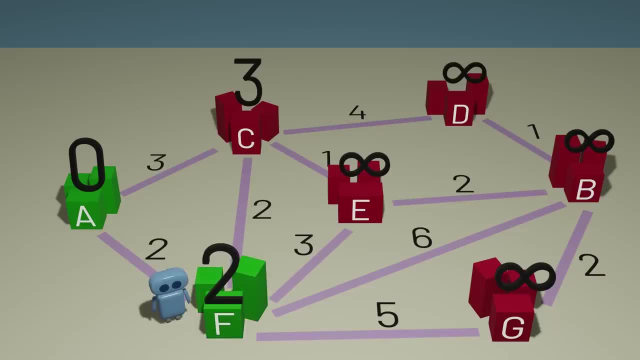 which we can get to in two minutes. And now the two-part process of Dijkstra's algorithm repeats. We first update our estimates by looking at the towns connected to town F. It takes five minutes to get from town F to town G. 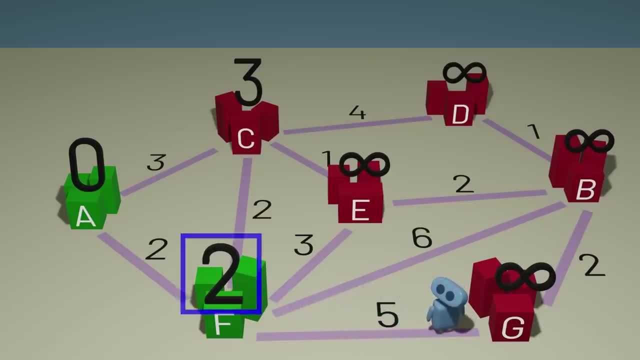 so if we can get to town F in two minutes, then we can get to town G in seven minutes. the sum of those two values. Likewise, we can get to town B in eight minutes and we can get to town E in five minutes. 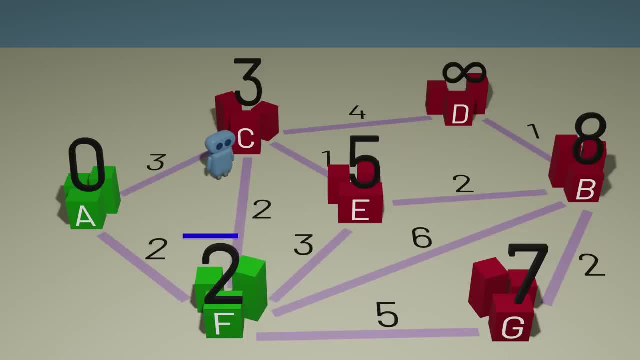 We can also get to town C in four minutes. two minutes to go from A to F and then another two to go from F to C. But four minutes is actually more than our current best estimate for town C, which is three minutes. 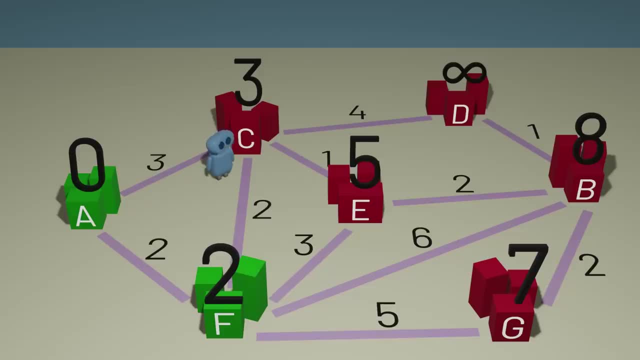 So we don't want to update anything here. Remember, for each town we want to store our best estimate for the shortest amount of time required to get there, So let's keep going. The second part of Dijkstra's algorithm tells us to explore the unexplored towns. 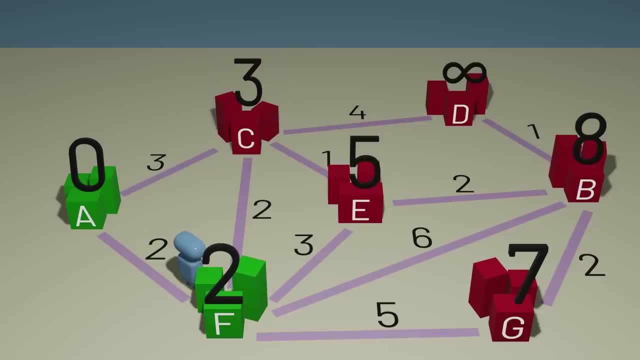 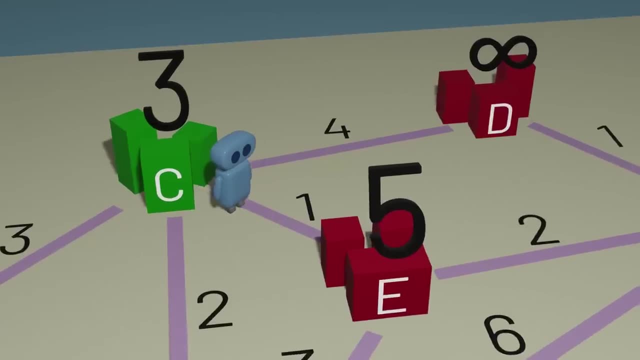 with the smallest value, And in this case that's town C, which we can get to in just three minutes, And the process repeats again. Going through town C, we can get to town D in seven minutes, and we can also get to town E in four minutes. 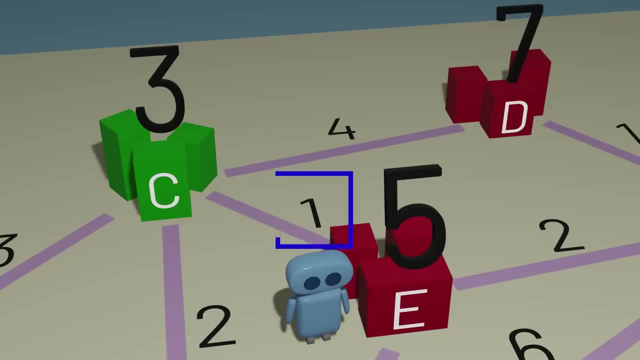 three minutes to town C plus one minute from C to E. That four-minute estimate is better than our current estimate of five minutes, so we'll update our estimate for town E from five to four. The next town to explore is town E. 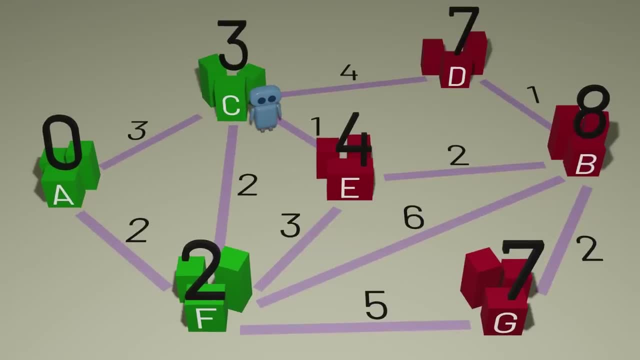 Among all the unexplored towns, it has the smallest value. Notice that each time we explore a new town, it's guaranteed that we will have found the shortest path to get to that town, since if there were some shorter path, we would have explored that shorter path first. 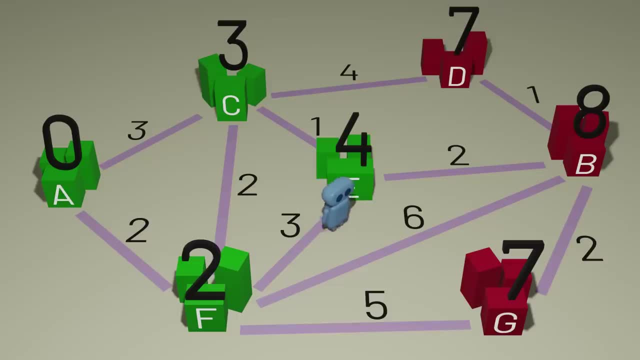 because we prioritize exploring the smaller values And through town E we can get to town B in just six minutes. four minutes to town E plus two minutes to go from E to B. So we update our estimate for town B to be six. 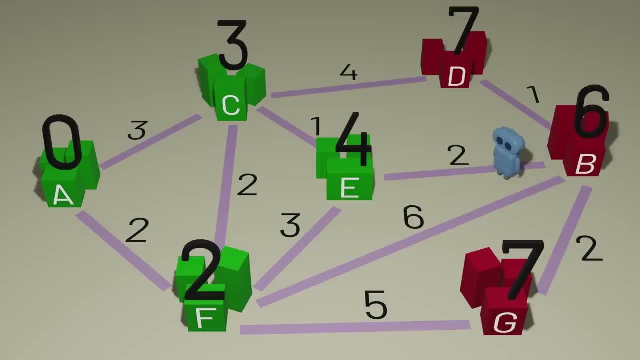 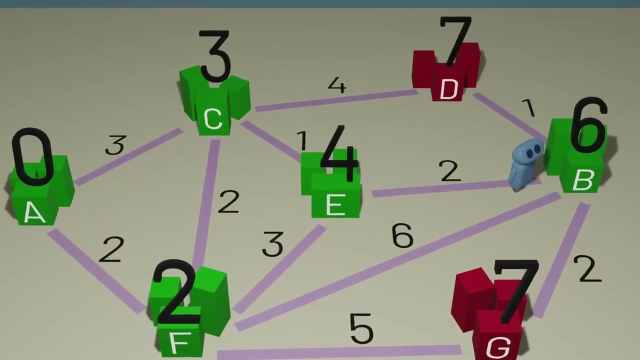 which is better than the previous estimate of eight. And now the next town to visit is town B, our destination, And that tells us that the shortest time needed to get from town A to town B is therefore six minutes, And that's Dijkstra's algorithm. 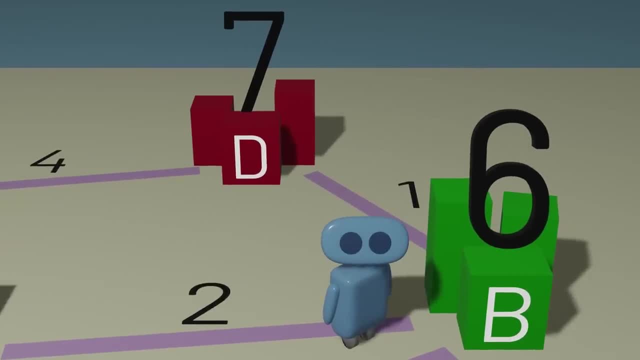 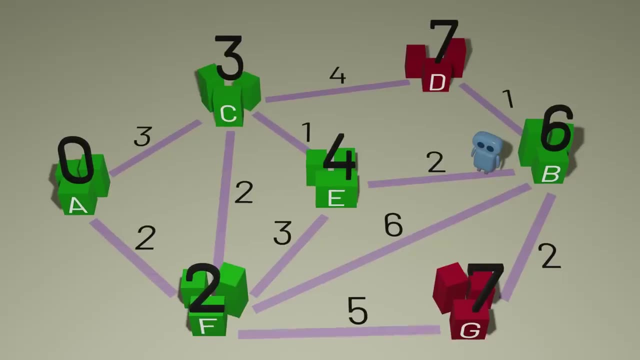 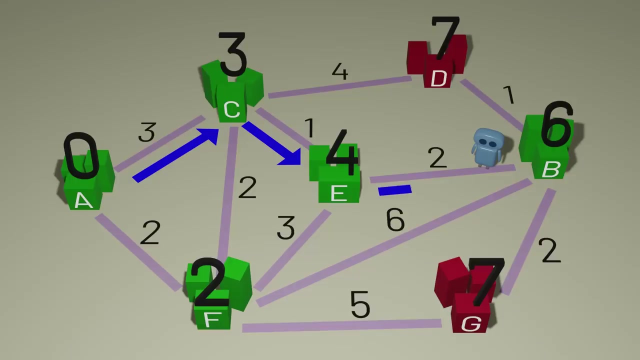 for finding the shortest path in a graph. Now, there are a few things worth pointing out here. The first is that, technically, our algorithm has only given us how long it will take to get from town A to town B, and hasn't actually given us which path to follow. 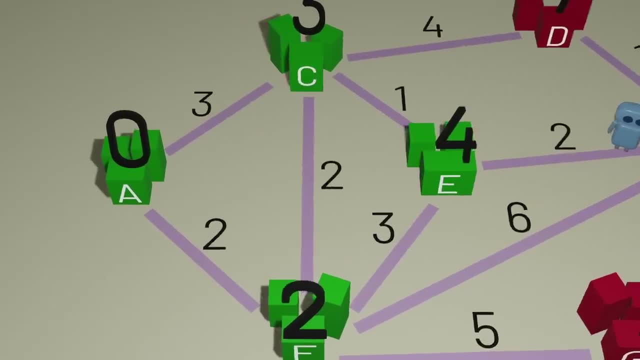 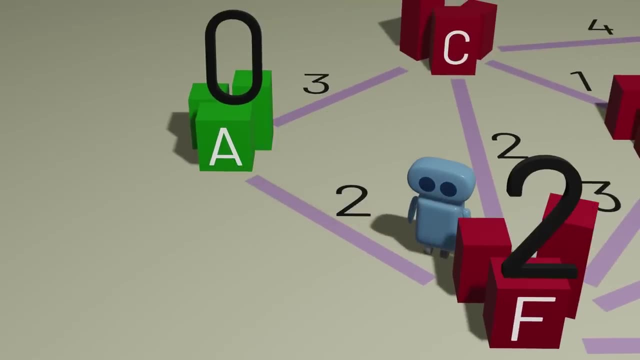 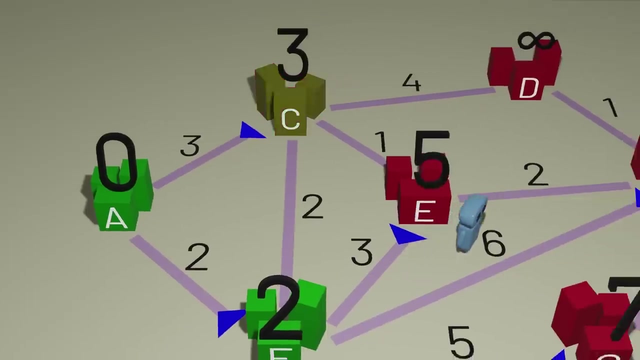 In order to actually reconstruct that path, we'll need to add a step to our algorithm. Every time we update our estimate for a town, we should also keep track of what previous town we visited in order to get to this new estimate. If we keep track of that for each of the towns,